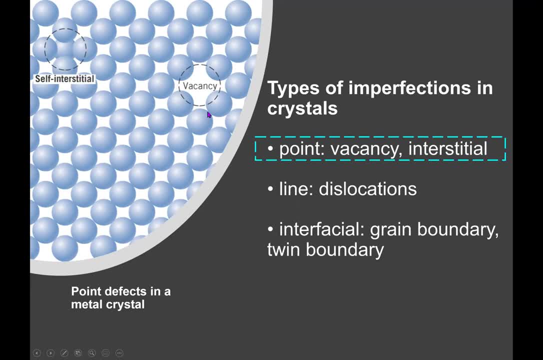 And now we can see that there's a missing atom. So missing atoms are simply referred to as vacancies in the structure, And we could also have the case where maybe an atom exists where it shouldn't, So it's imbued, So it's an interstitial that exists between atoms like this one here, and this is referred to as an interstitial. 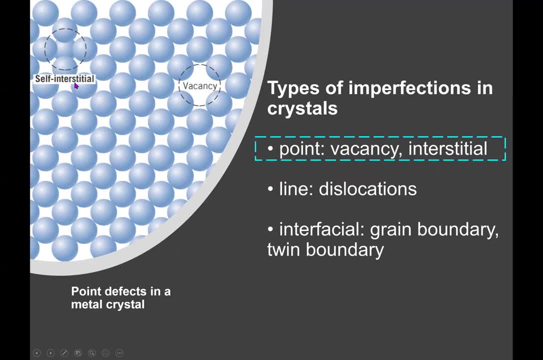 These sites between the atoms are referred to as interstitial sites. This one, specifically, is a self-interstitial because it's an atom of the same type. We could also talk about impurity interstitials, which would be an atom of a different type into this lattice. 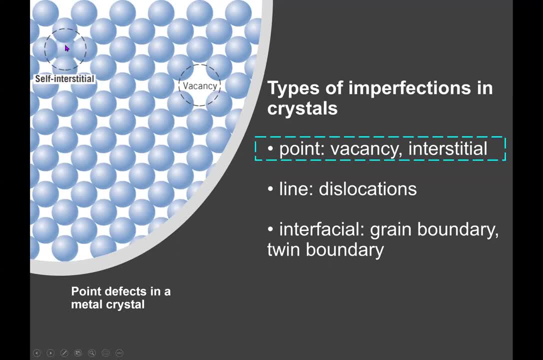 All right. so one thing you can see about a self-interstitial is that it's not going to fit. So, the way this is drawn, these atoms are all overlapping, So this lattice would have to stretch out and distort in order to fit this atom right in here in this site. 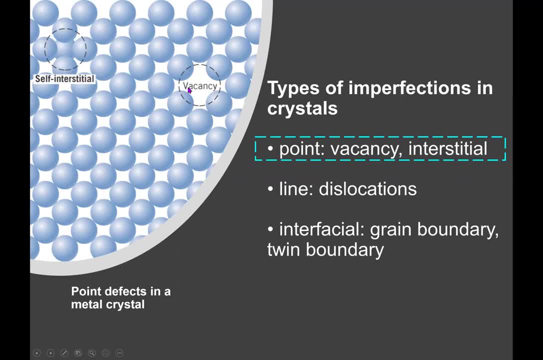 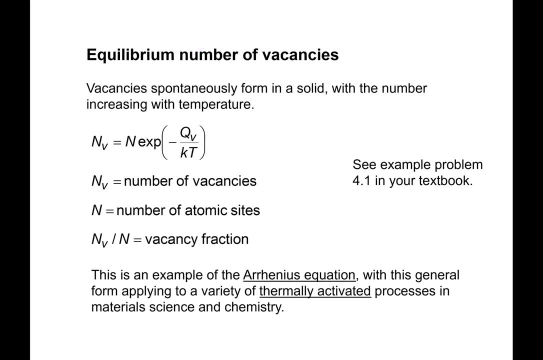 So this is not going to be as common as, say, a vacancy. The vacancies are one of the defects that are actually thermodynamically stable, So we can't get rid of them. In fact, there are a number. There's an equilibrium number of them that depends on the temperature of the solid. 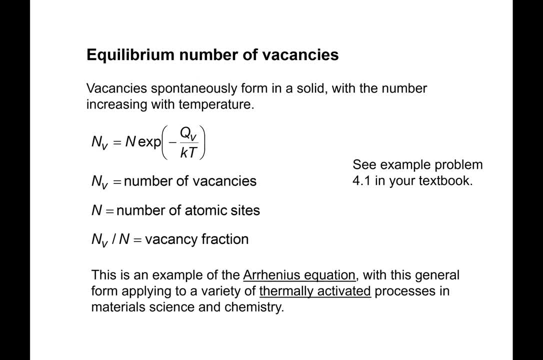 And as we approach the melting point, this number of vacancies increases exponentially. So you'll have a problem in your homework. Take a look at the number of vacancies in a solid. I'll just refer you to problem 4.1 in your textbook, which will run through a simple problem using this equation. 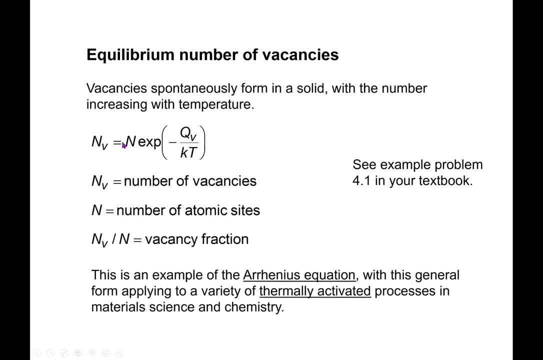 But let's take a look at the equation for a second. This is called an Arrhenius equation. Anytime you see an equation of this form, we've got an exponential of some kind of an energy barrier over kT, That's thermal energy. 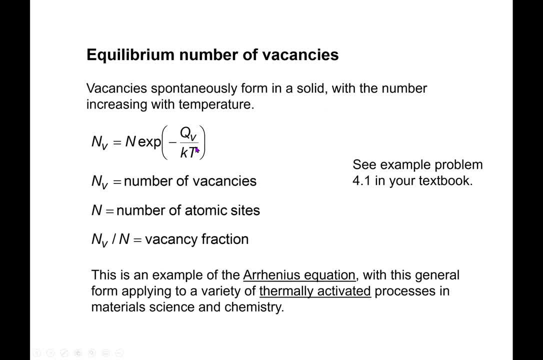 This Boltzmann's constant And this is the temperature in Kelvin. So this is like a probability that we can overcome this formation, energy or this barrier. You've seen this before in chemical kinetics, where this was the energy for a reaction to overcome the barrier. 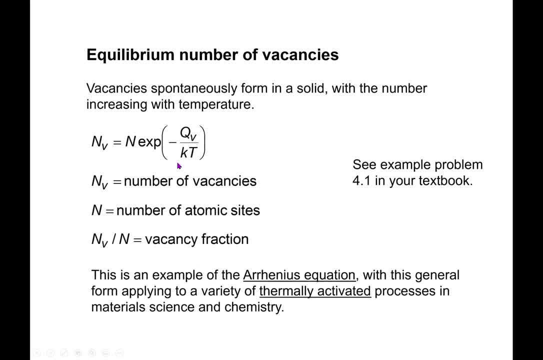 So this is like a probability that a given site could be a vacancy And then this is the number of sites that are in our given structure, say per meter cubed, And then that will give us the number of vacancies in that same volume, say meter cubed. 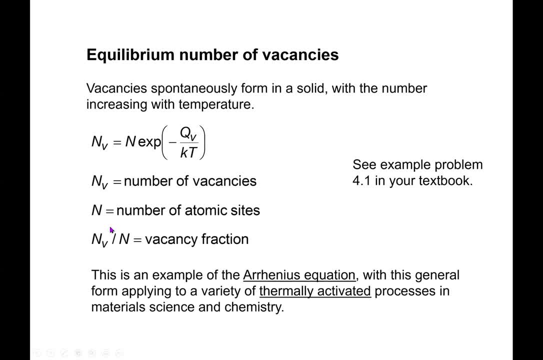 So many times. we'll just move this n over here And we'll look at simply the vacancy fraction, So the number of vacancies per atom site in a given material Vacancy fraction. All right, Let's see what else can we say. 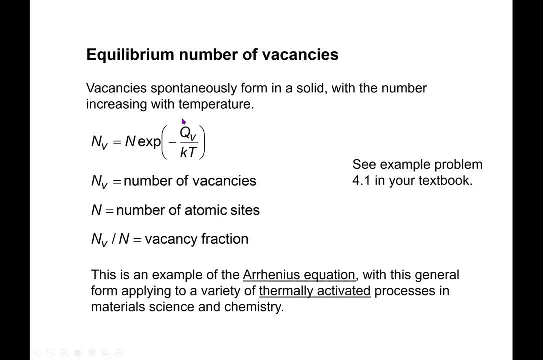 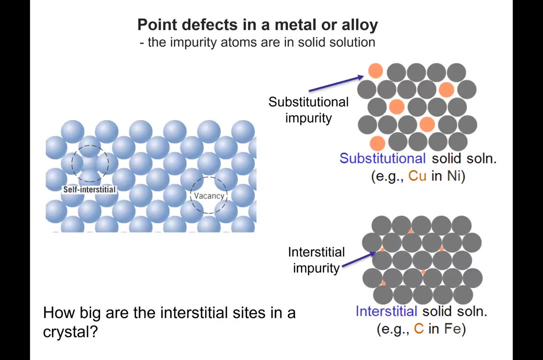 This activation energy Q we're going to see is on the order of an electron volt, So that's a convenient unit to use. So you're going to need to use Boltzmann's constant also in units of electron volts. All right, Point. defects in a metal or alloy continued here. 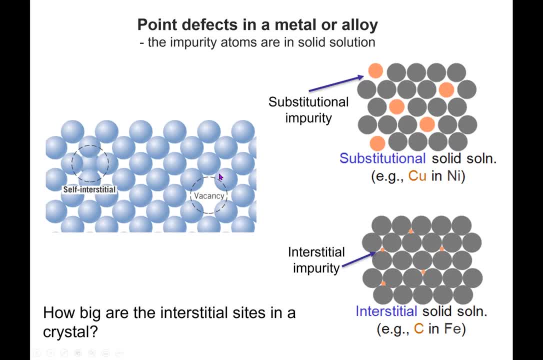 So we've seen the self-interstitial And we've seen the vacancy, the missing atom case. We can also talk about these defects when we also have alloys. So let's say we had an alloy here, maybe of nickel, So we have a crystal structure here of nickel. 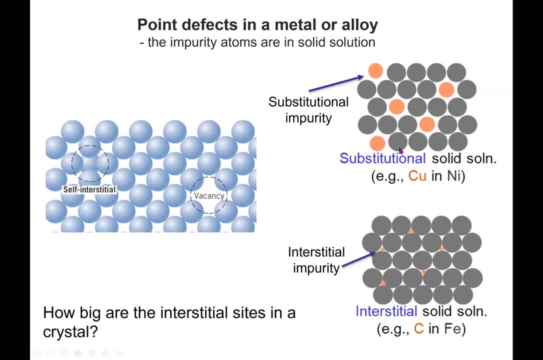 This is a face-centered cubic material, So this represents maybe 1, 1, 1 plane. And then we're substituting in copper in place of some of the nickel in this lattice, These atomic sites. So this is a substitutional impurity. 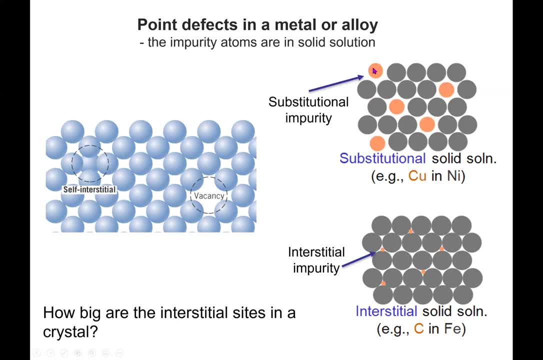 I'm removing the host atom, I'm substituting in a different type, So it's substitutional impurity And this alloy is referred to as a substitutional solid solution. Now we could also take an alloy, a smaller atom, into a host and have it locate at interstitial sites. 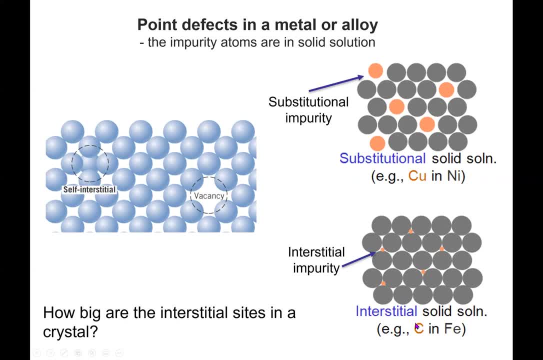 It's referred to as an interstitial impurity. A good example of this one would be carbon in iron forming a steel. So we'd have a steel structure, the iron the host, and then the carbon would sit in the interstitial sites. 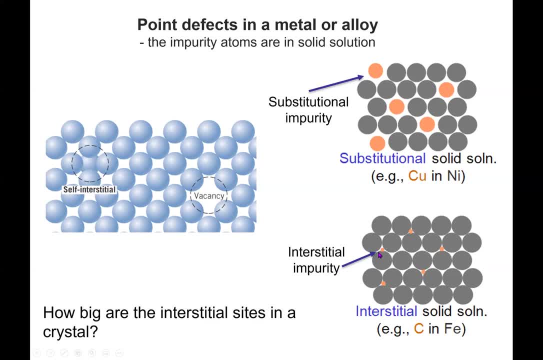 Okay, Now in this picture it makes it look like it sits perfectly in here. In fact, the carbon is a little bit big, And so it does distort the lattice, increases the energy of that system, And so we'll see that we can't put a whole lot of carbon into the iron because of this. 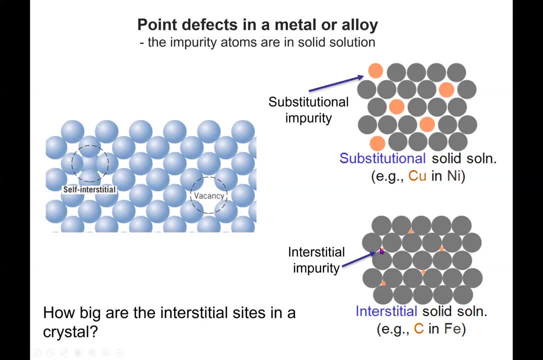 If you try and push in too much, then the carbon will precipitate out of this lattice and form an iron carbide. All right, So what we want to do is to go ahead and see if we can calculate, with our knowledge of crystal structures, what the size of these interstitial sites might be. 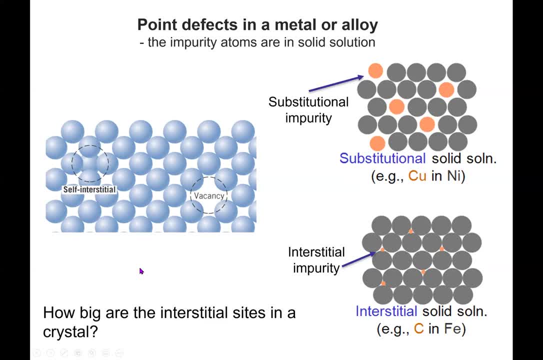 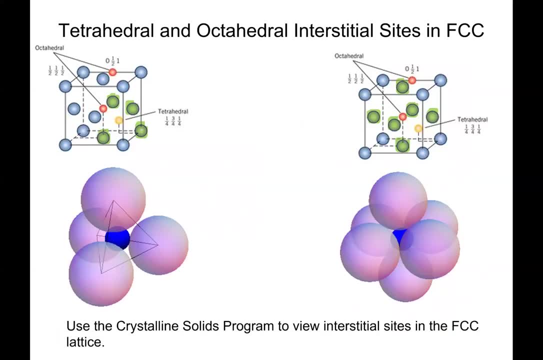 So we're going to take a look at the types of interstitial sites we have and then see if we can calculate their size. So I'm just going to define two types. in the face-centered cubic structure, your book will describe for you the body-centered cubic structure. 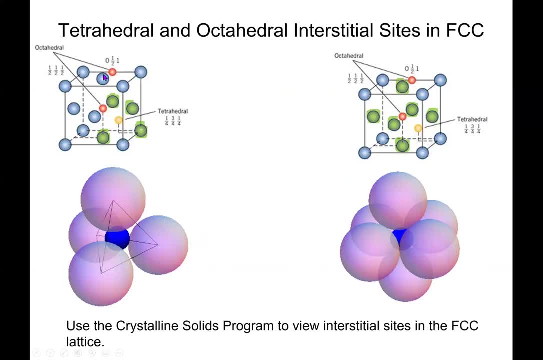 Okay. So if we take a look at the face-centered cubic structure, so these atoms here in blue- and I've highlighted a few of them here and talk about that in a second, But the blue are in face-centered cubic positions- Okay. 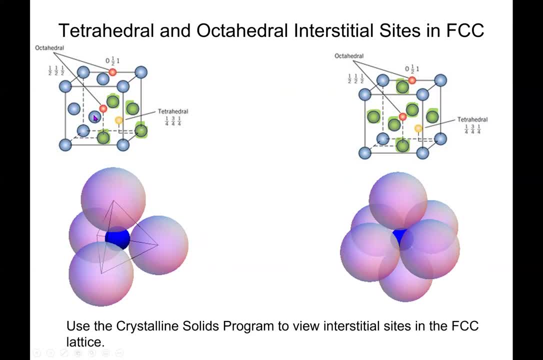 You can see the centers here are faces containing the blue atoms, And then they've got a couple of other atoms, impurity atoms, that are located in between sites. So there's one that's directly in the middle And I'll talk about that one in just a second over here. 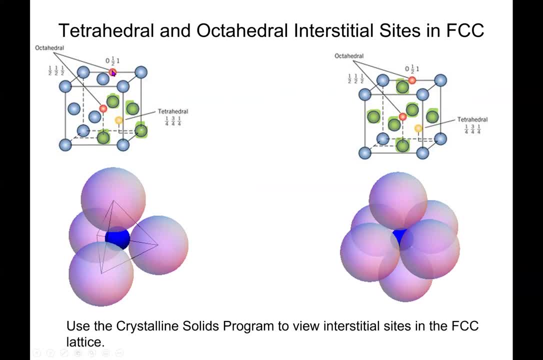 We've got one sitting on this edge, Okay, So that represents a type of site that could be any of the edges, And we've got one that's sitting here that we've seen before in the diamond cubic structure, the zinc blend structure. 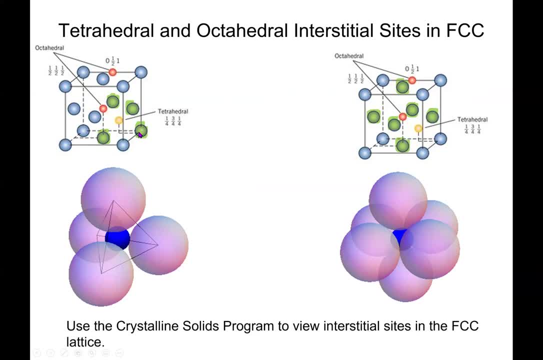 That's sitting off of this atom by a quarter, quarter quarter in terms of its location, And this one is the one that is in a tetrahedral site. So if I take this corner atom and the three faces, neighboring faces, we will find that these three form a triangle. 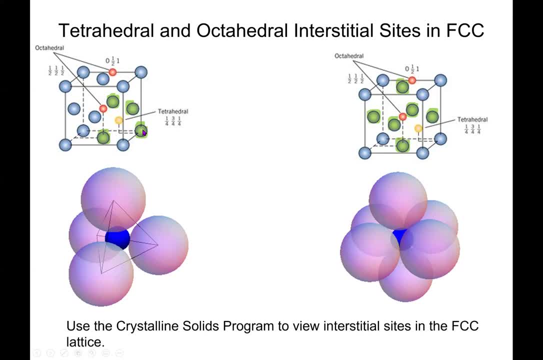 They're all touching, And this one's sitting on top of them, also touching, And so here's our picture. So if you want this atom, is this one here? This is our little tetrahedral atom sitting in the middle in this tetrahedral site. 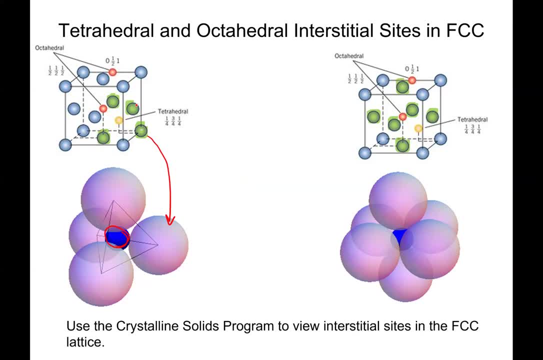 Okay, And then we've got these other three atoms forming this base of this pyramid, And so we want to find out what the size of this atom is that just fits in this little tetrahedral site. Okay, The one in the center. if I look over here, there's a big hole in the face center cubic structure, right in the center of the body. 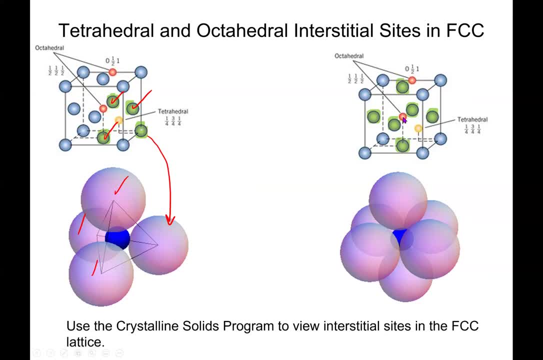 And you've got to position one half, one half, one half, And if I take the neighboring six face atoms, those are actually all touching. You can see that down here. And then there's the site right in the middle And this is referred to as an octahedron. 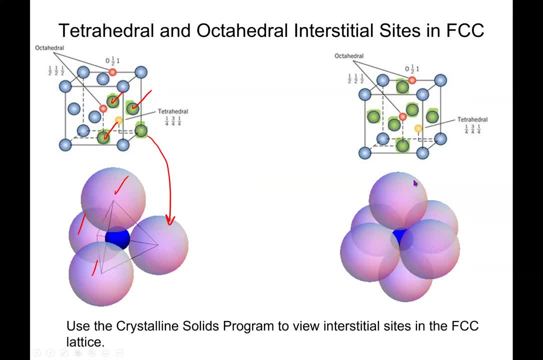 I connect all these sides. You can see here this forms an octahedron. So this is an octahedral site, All right, And a similar kind of site here for the edges. If we were to put on the rest of the blue lattice, we'd actually see that this is similar. 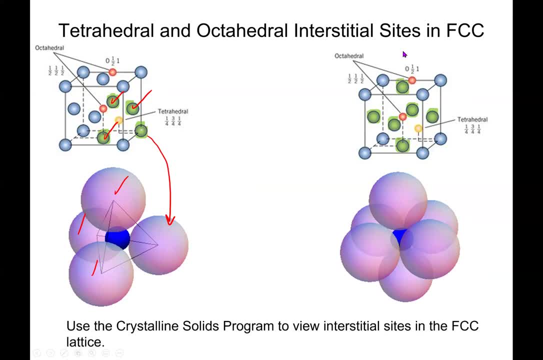 And again it forms an octahedral site. So for homework you're going to have to work on this one, the octahedral site. I'm going to go ahead and show you how to do this tetrahedral one so you can use the same method for the octahedral. 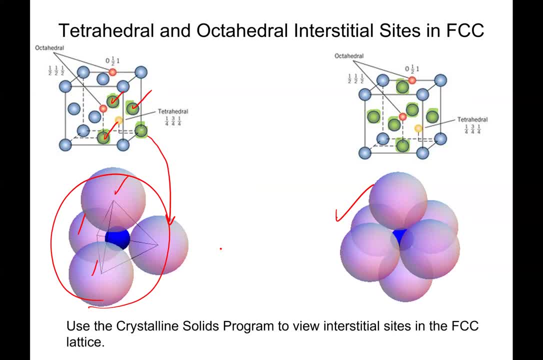 All right. So we could use a lot of geometry if we wanted And figure out the size of the spacing in here, But I'm going to try and show you just a simpler way, just using distance between points. This is essentially related to a dot product. 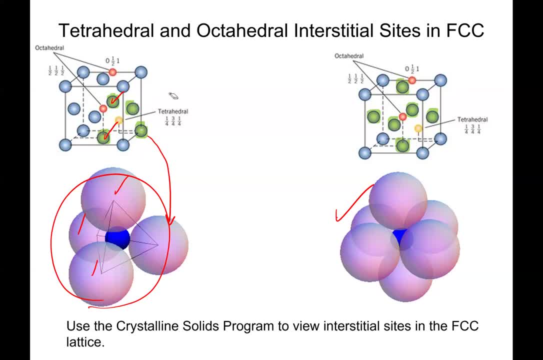 What I'm going to do is I'm going to go ahead and take this tetrahedral atom which is located at one quarter, three quarters, one quarter. You can see that's given. So that's given the problem, And I need one more atom that's touching it. 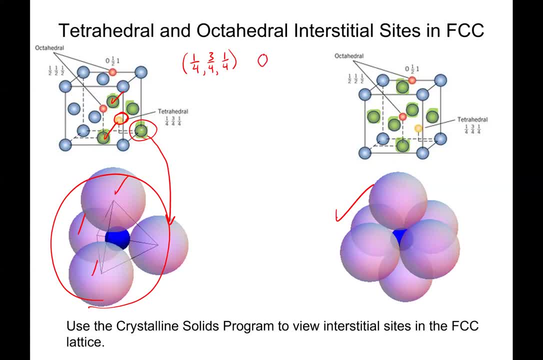 So I'm just going to go ahead and take this corner one here. It's easy for us to get a coordinate from. So that's 0, 1, 0.. All right, So let's go ahead and subtract these two. 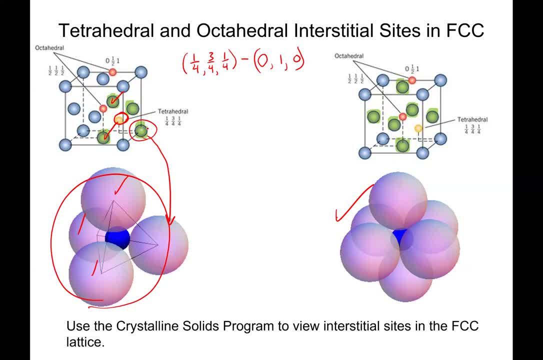 So that'll form the vector connecting these two points. So that would be a vector be one quarter, three quarters minus one is minus quarter a quarter and the magnitude of that. so that'll be now the distance between the tetrahedral atom and the corner atom. it's going to be square root of 3 over 4. so let me go. 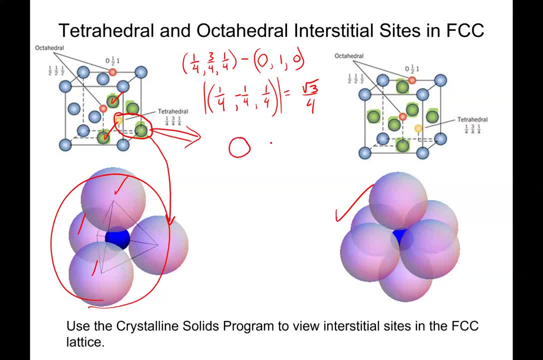 ahead and we'll grab these two atoms and see what we just did. so I've got that one, I've got this big one they're touching. this is little R in the center, here is big R, and so what I do know is that distance between these now is. 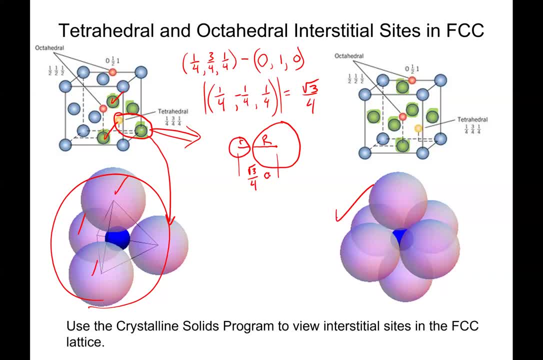 square root, 3 R. but I have to remember that I need to multiply by this a, because this work up here was done relative to the edge length of our unit cells is just fractional. but if I want to actually start putting the size of atoms into this structure, then I want to use the real dimension. so I'm going to 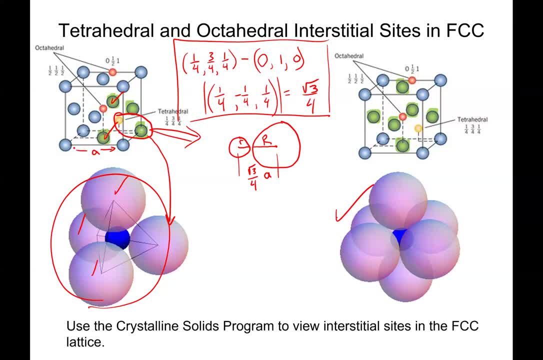 multiply by a the length here, so I can get real coordinates. so what I have then is little R plus big R. here is equal to the square root of 3 over 4 times a, and you'll recall that for the face centered system. I hope that the edge 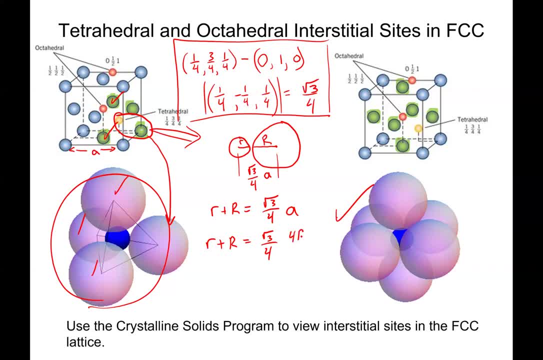 length a is given by 4 times the radius of the host here over the square root of 2. all right, so if we just go ahead and rearrange, I'm going to get our little R over. R is equal to the square root of 3 over the square root of 2 minus 1 put.